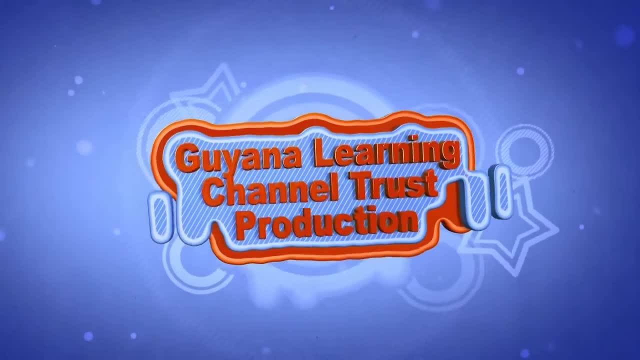 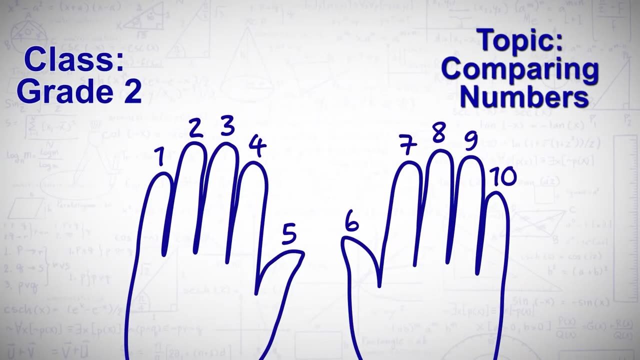 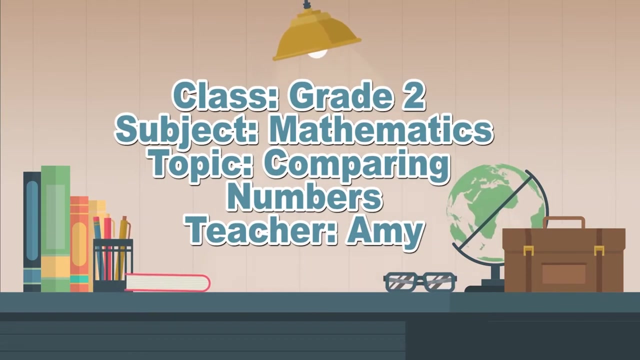 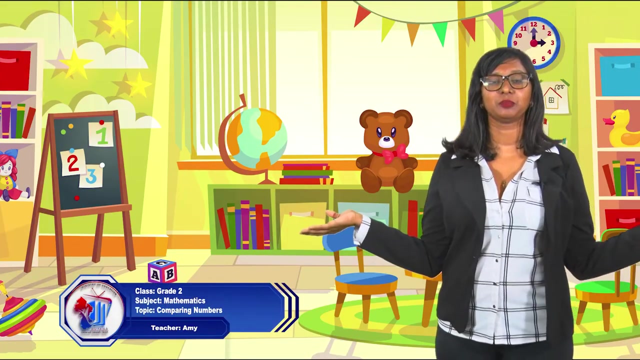 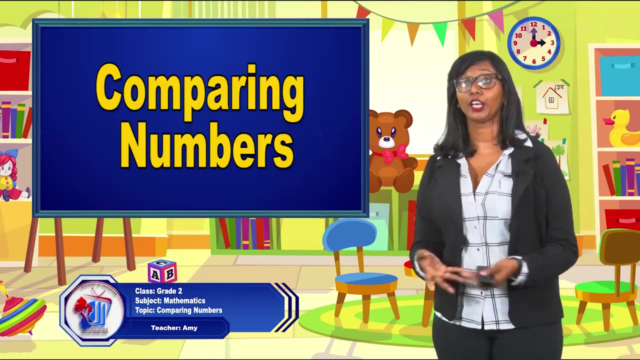 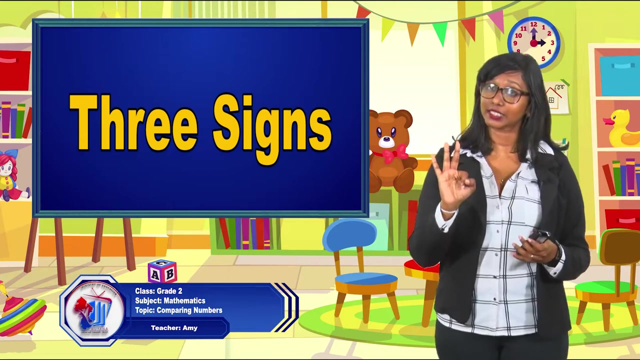 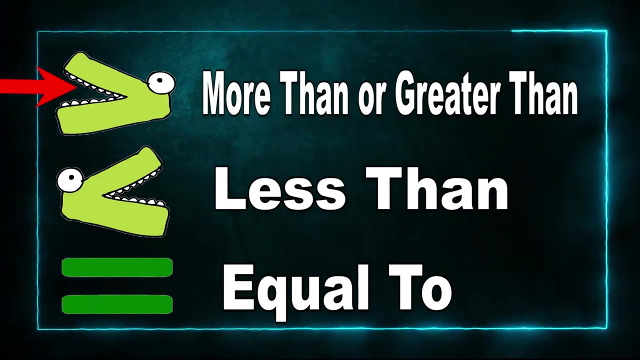 Hi there, boys and girls, and welcome to mathematics class. I am Miss Amy and today, for mathematics, we are going to be comparing numbers. Now, to compare numbers, we are going to use three signs. We have the more than sign or greater than. We have the less than sign and we have equal to. 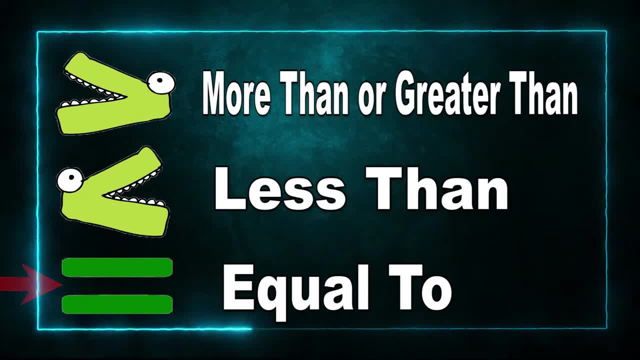 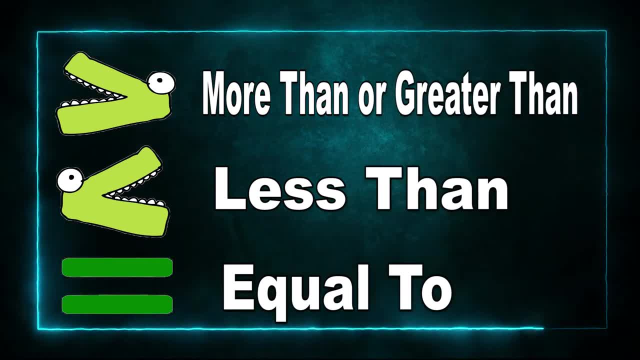 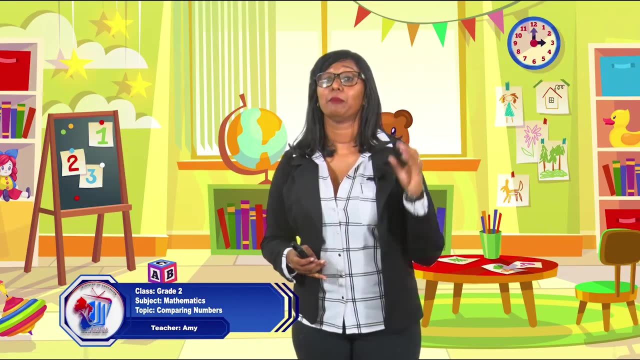 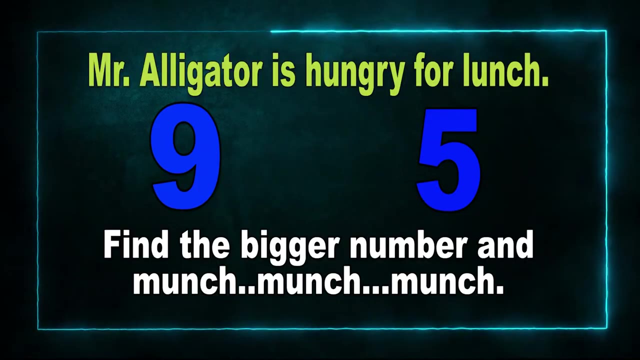 Now we can make this lesson very fun. Let's call our more than sign and our less than sign an alligator's mouth. Now, an alligator is always hungry, So the mouth of the alligator will always go towards the bigger number. So let's take a look here. 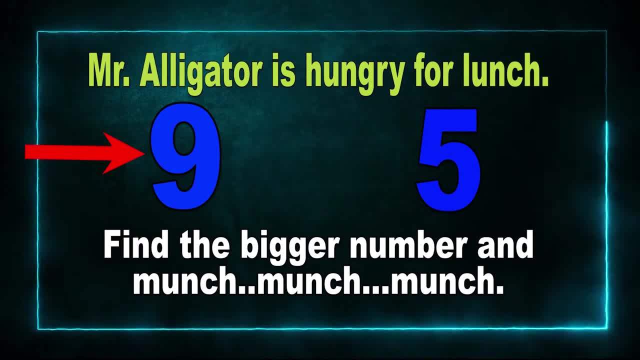 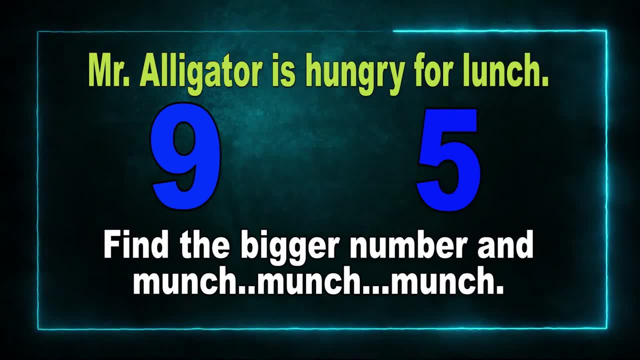 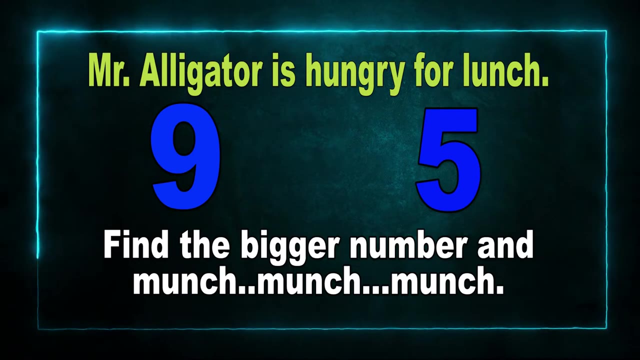 We have nine And we have five. Mr Alligator is hungry for lunch, So he is going to find the bigger number and munch munch. Now let's take a look. We have nine and we have five. Which one of these numbers do you think he is going to munch on? 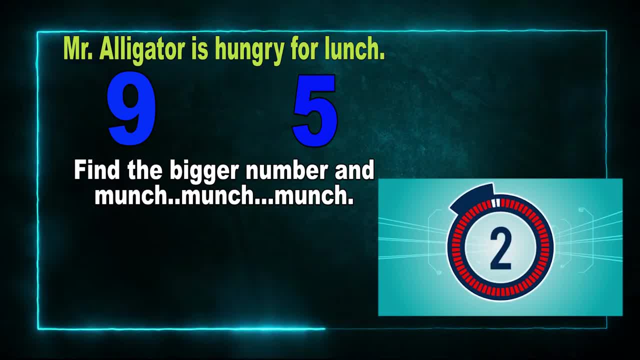 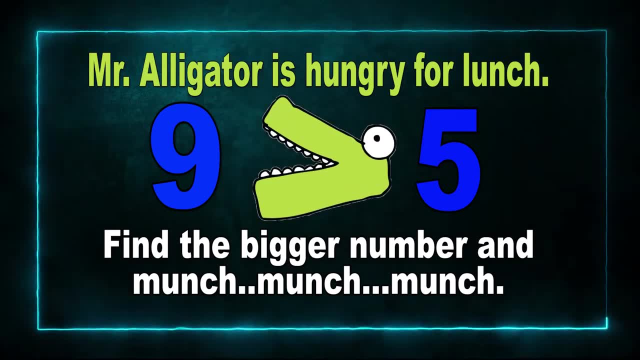 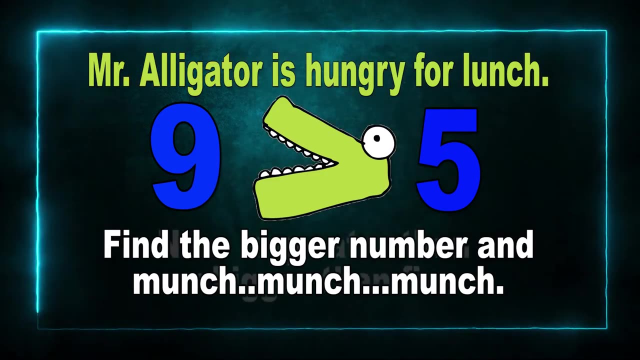 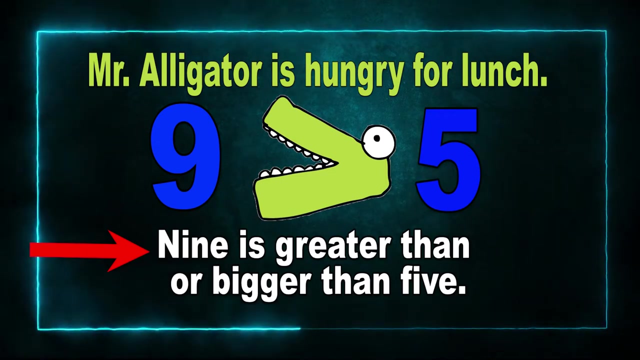 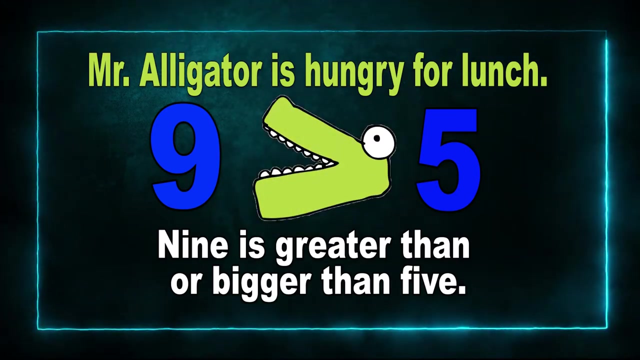 He will munch on nine, So the mouth of the alligator will be open to nine. To read this equation, we can say: nine is greater than or bigger than five. Nine is greater than or bigger than five. Now, remember, boys and girls. the mouth of the alligator will always be open to the bigger number. 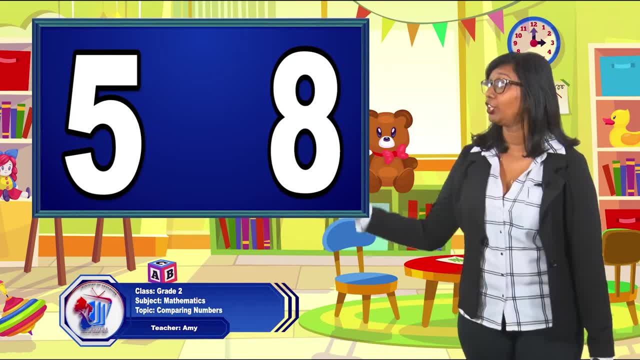 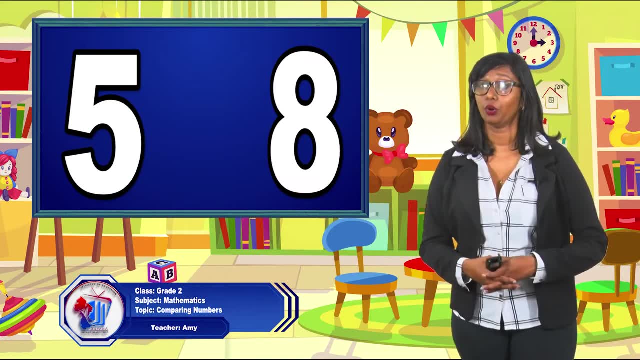 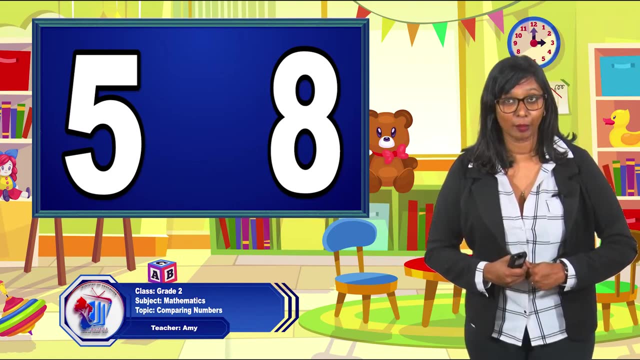 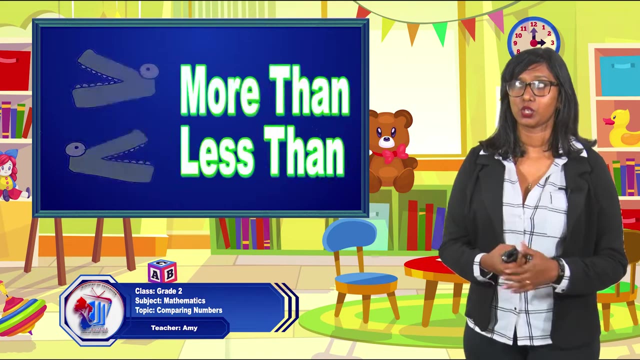 So let's take a look here. We have the number five and then we have the number eight. Now we want to know which number is bigger. So for us to compare these two numbers, we are going to use a sign. but with sign do we use? do we use the more? 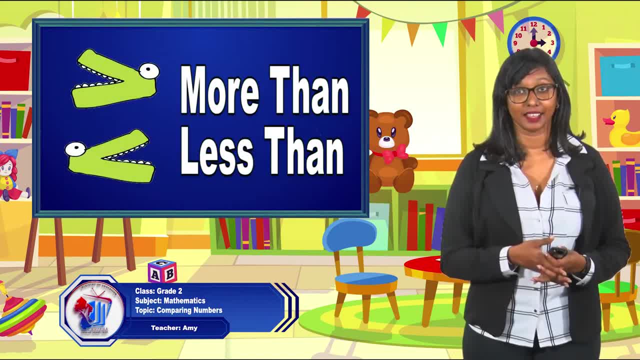 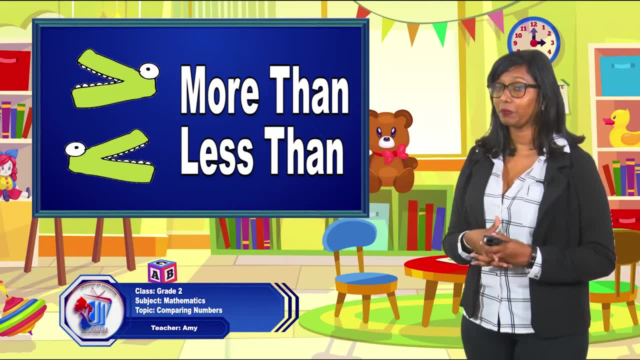 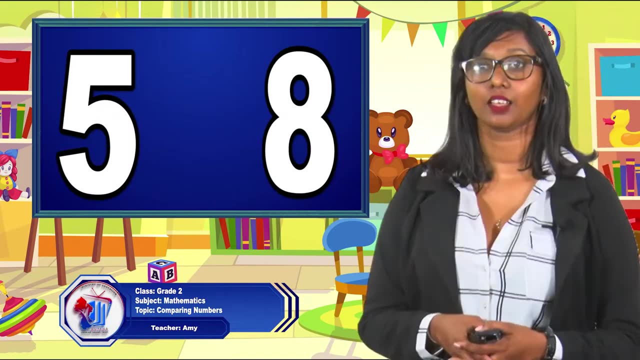 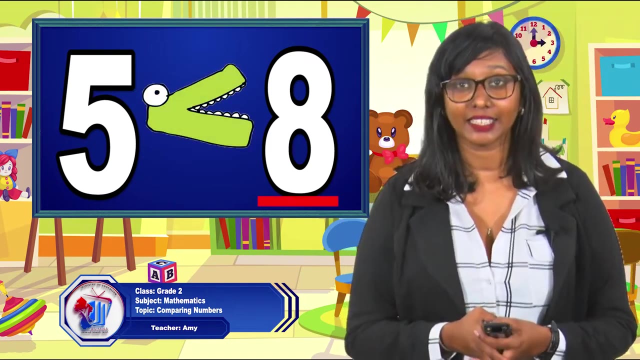 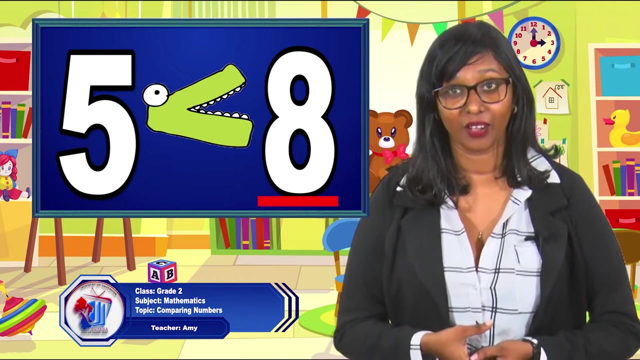 than sign, or do we use the less than sign? now let's take a look. remember, the alligators mouth will always be open to the bigger number. so let's take a look. five and eight, which number is bigger? the number eight. so the mouth of the alligator will be facing it. so read this now. yes, we can read numbers too. to read: 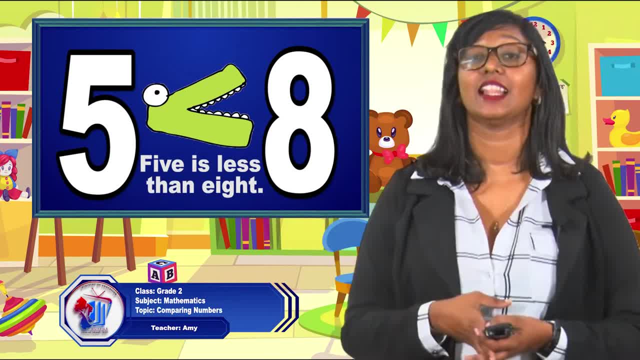 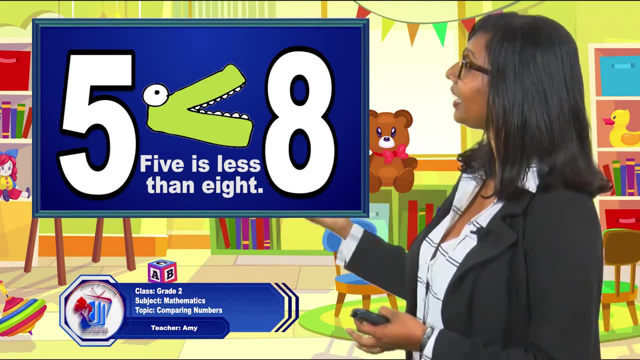 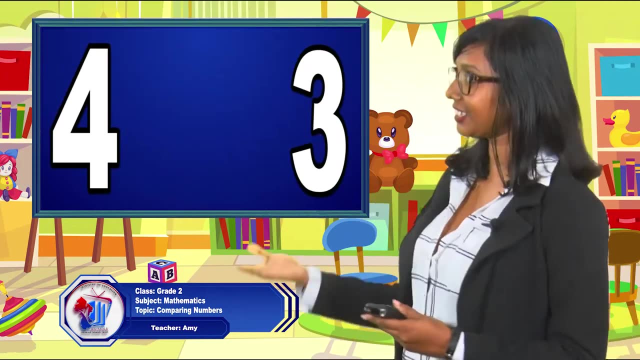 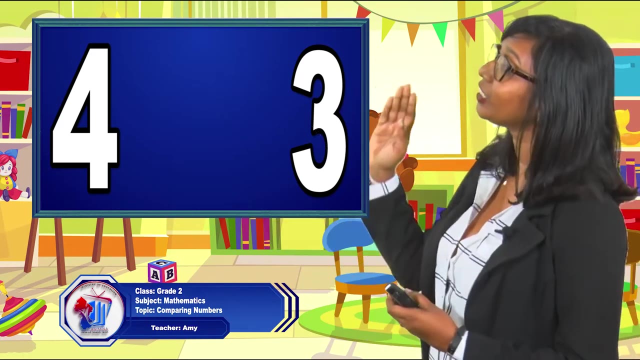 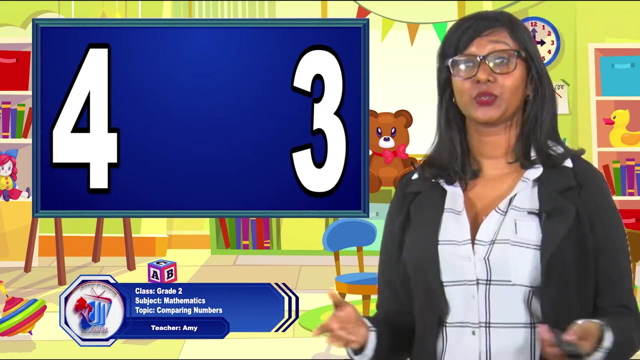 this. we say: five is less than eight, five is less than eight, five is less than eight, eight. okay, boys and girls, this is very easy, isn't that? so now, take a look at this. we have four and three. four and three. now we want to compare these two numbers we are going to use 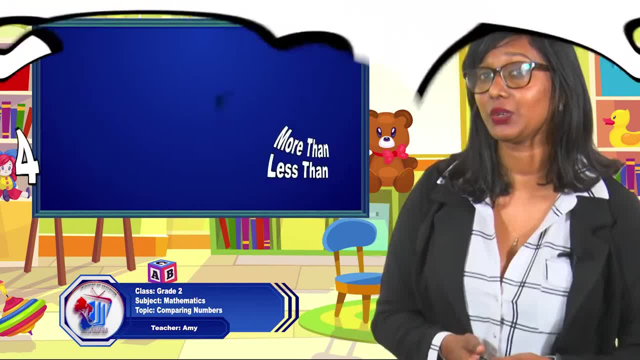 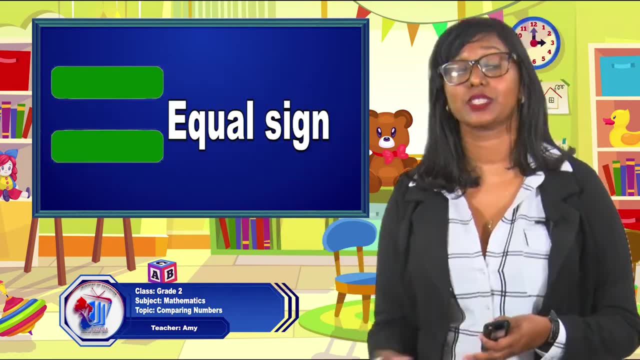 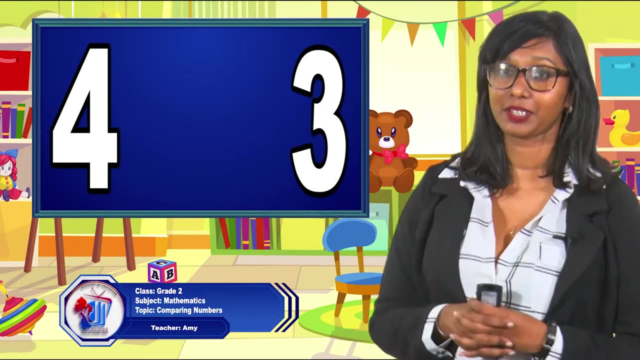 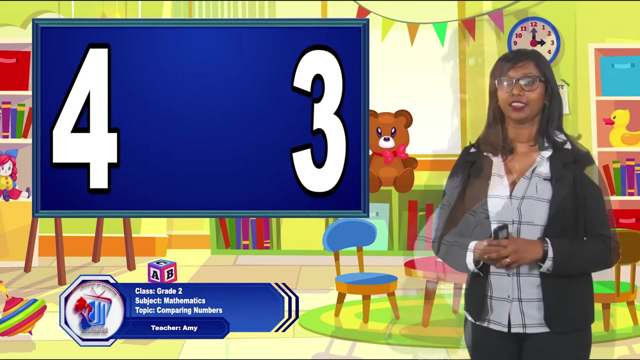 a sign. but which sign will we use? will we use the more than sign, will we use the less than sign or will we use the equal sign? now let us take a look very, very carefully at our numbers. remember, mr alligator is hungry, so he will munch on. the bigger number, so the bigger. 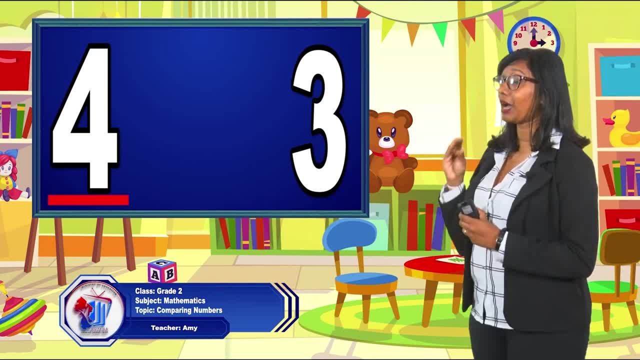 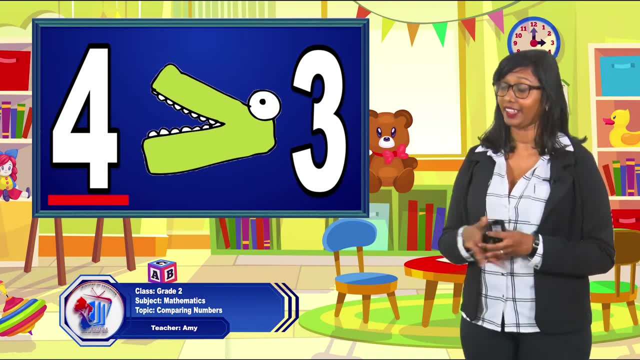 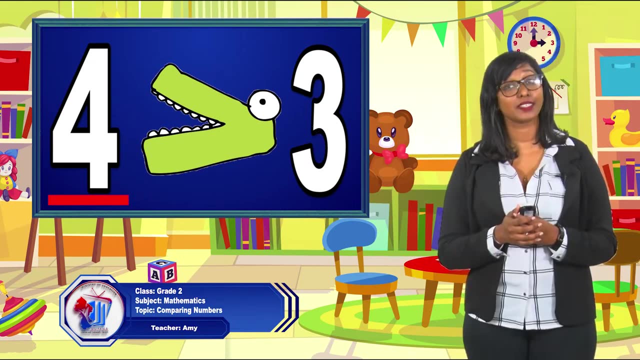 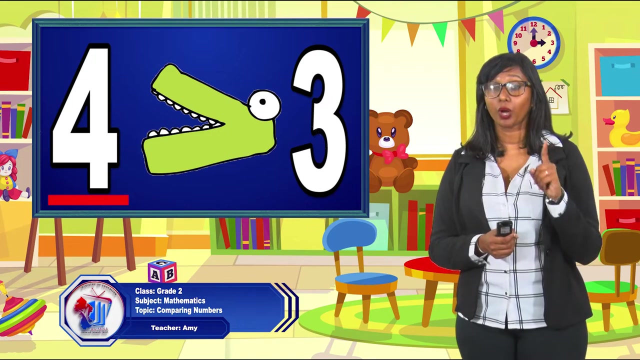 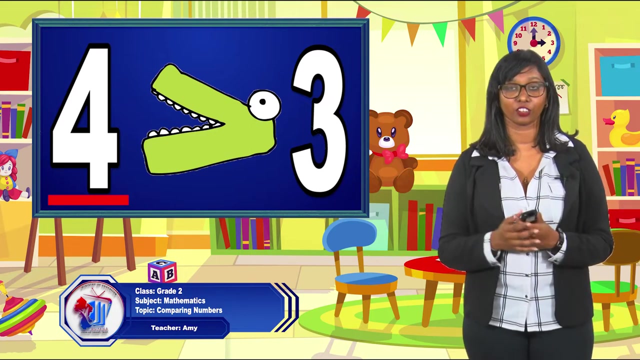 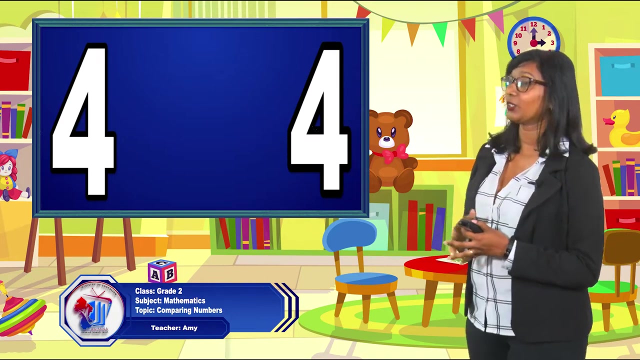 number is four, so the mouth of the alligator will turn to four. so to read this: we say four is bigger than three, or we can say four is more than three. and there's also one more way that we can say this: we can say four is greater than 3.. Okay, boys and girls, now let's take a look at these two numbers. They 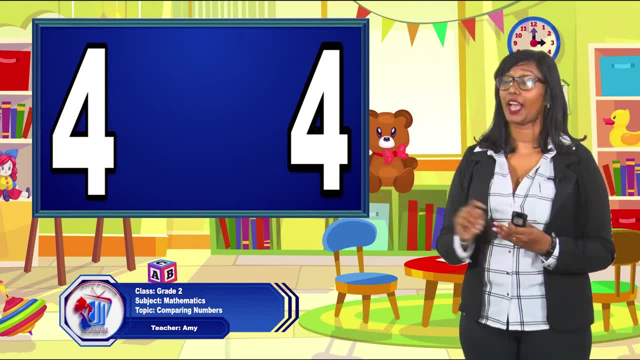 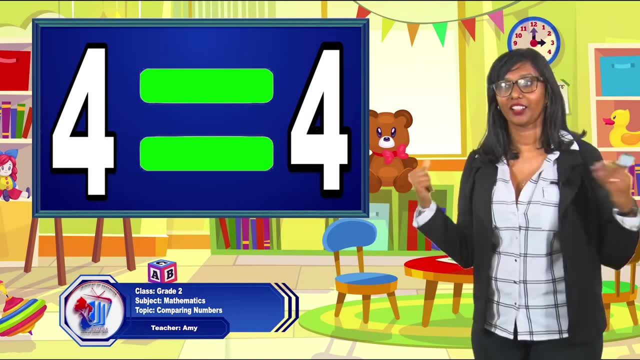 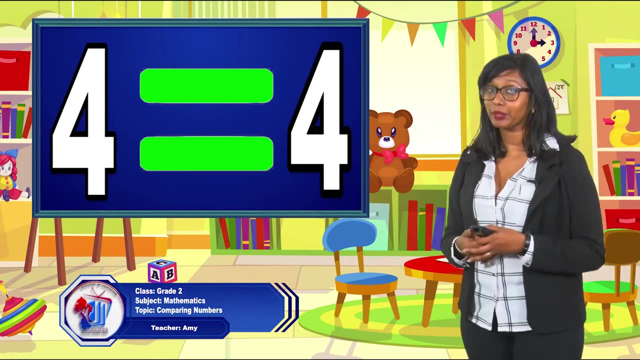 are 4 and 4.. We have 4 and 4.. They are equal. Very good, They are the same. We use our equal sign when the two numbers are the same. When they are the same numbers, we use our equal. 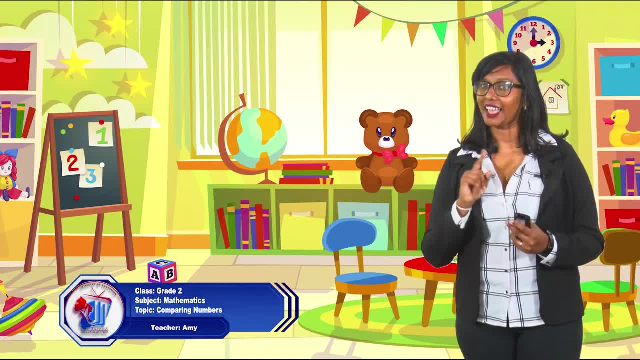 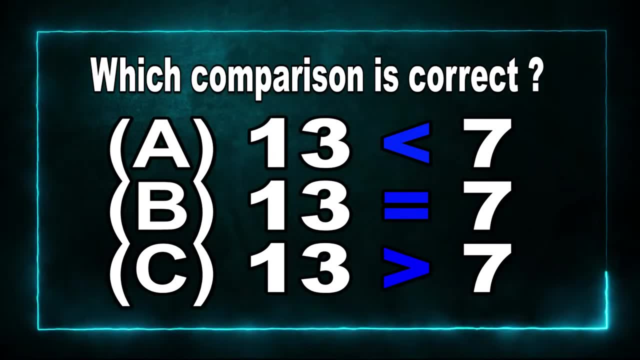 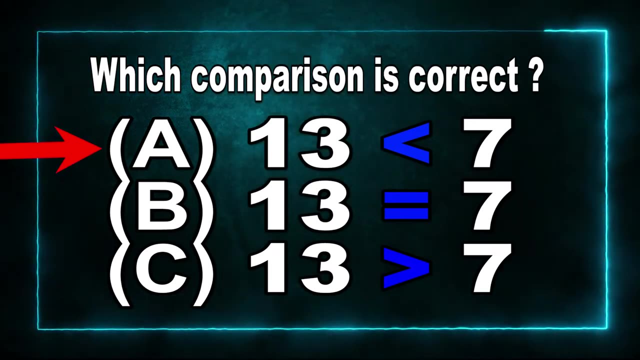 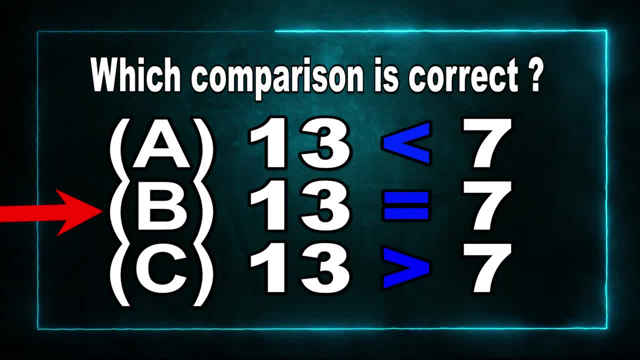 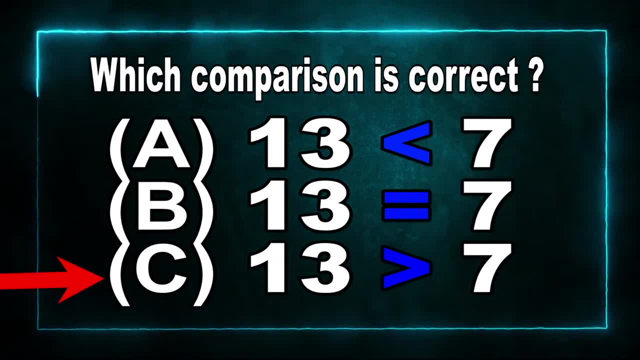 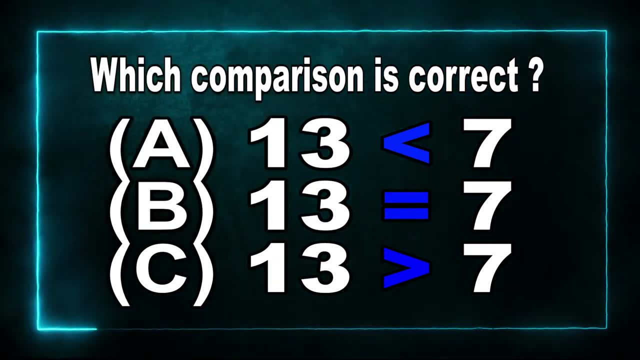 is equal to 7. And then we have: 13 is greater than 7.. Now remember, in order for us to use the equal sign, the two numbers have to be the same. Are these two numbers the same? No, they are not. 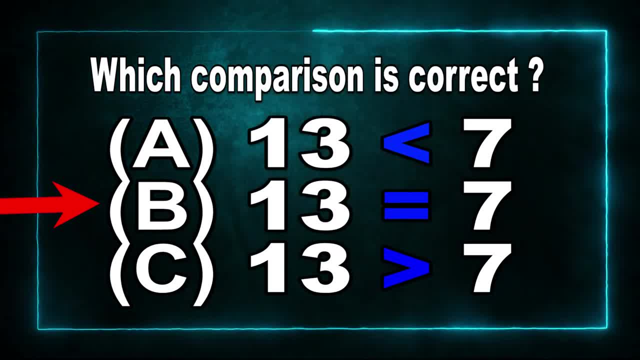 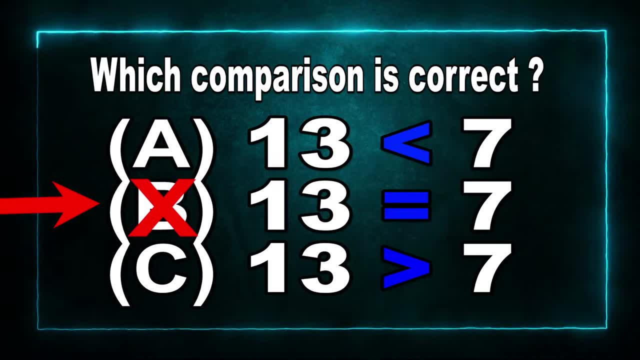 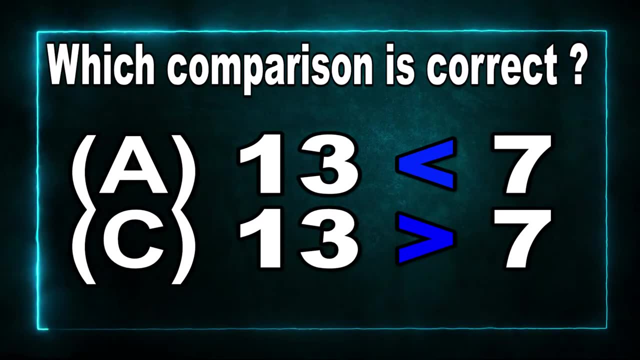 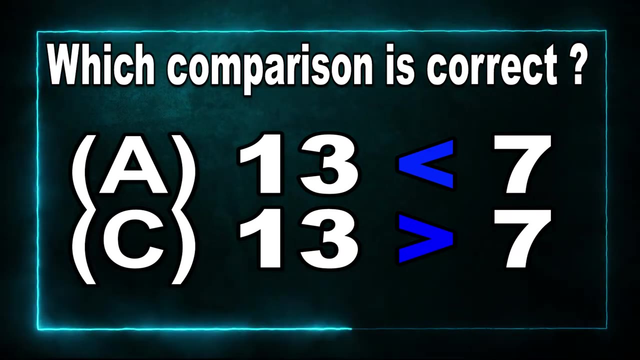 So we cannot use the equal sign. So therefore, letter B is wrong. That is not the answer, because the question says which one is correct. So let's look at letter A and letter C. Now. remember, Mr Alligator is hungry, so he wants to munch on numbers, and he will munch on the bigger number. 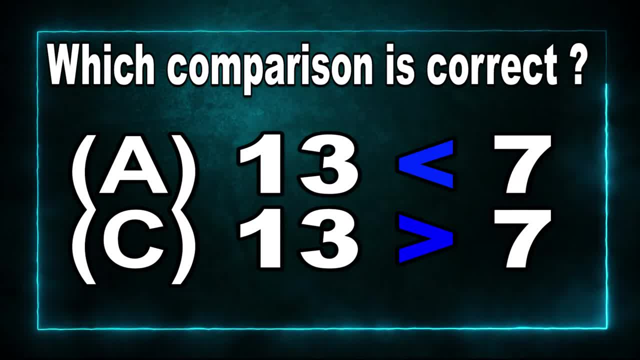 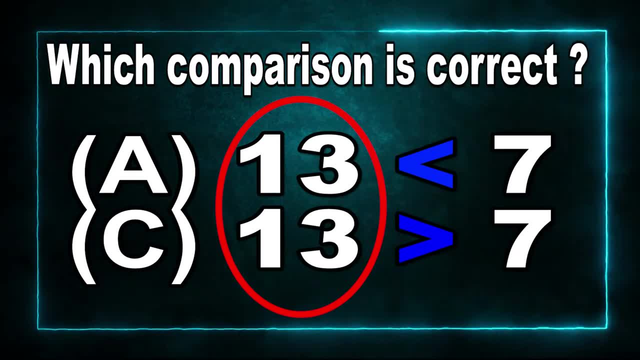 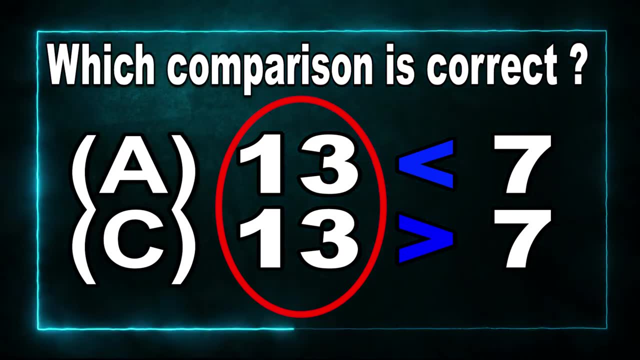 So 13 and 7. Which one is the bigger one? 13. 13 is the bigger one, so he will munch on 13.. So the mouth of the alligator will be open to 13.. Now take a look. letter A and letter C: 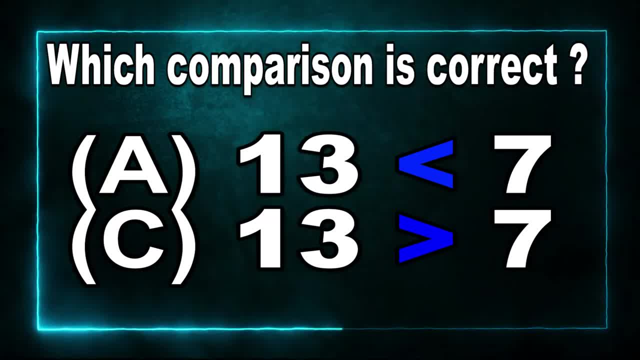 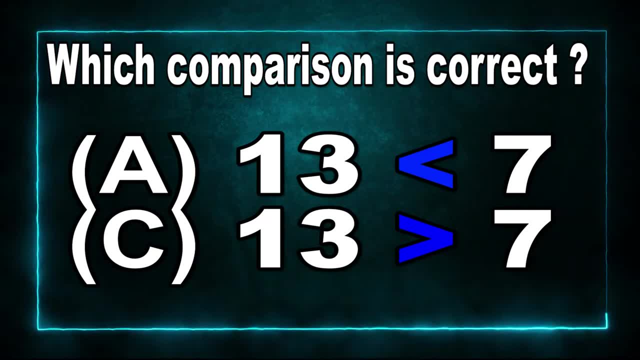 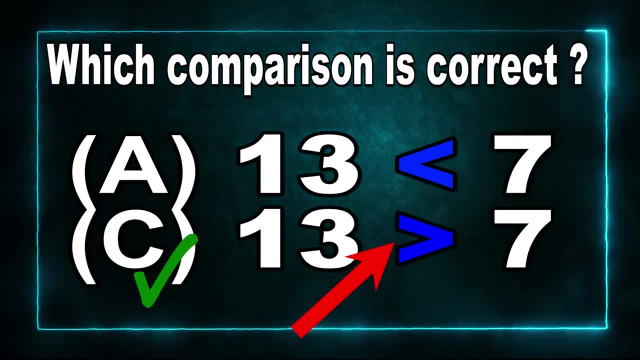 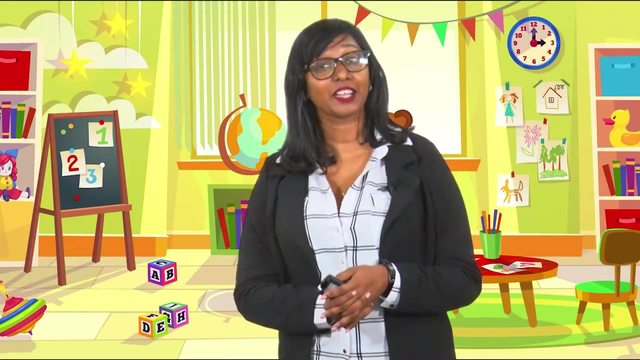 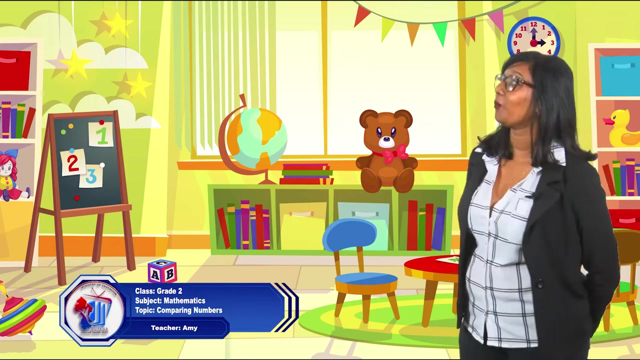 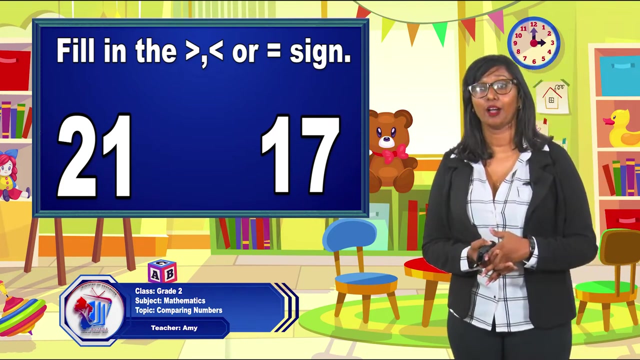 Which one of them there has the alligator mouth open to 13?? That will be letter C, The last one, The alligator mouth is open to 13.. So we can read: 13 is greater than 7.. Comparing numbers are easy, Isn't that? so So I have four here for you. I want you to put in the sign so that we can compare these numbers. 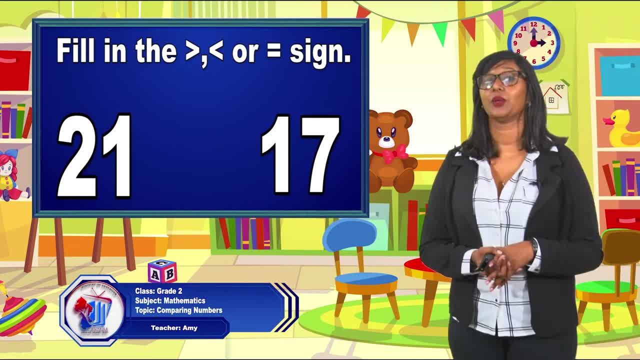 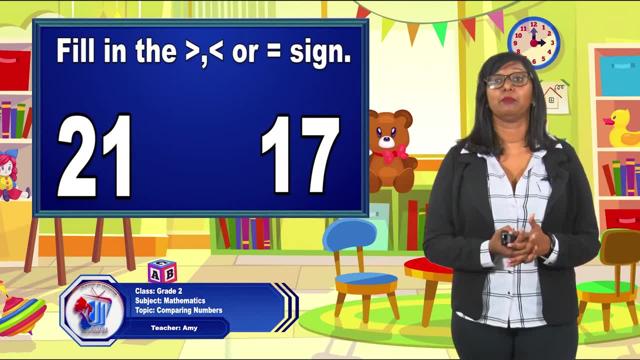 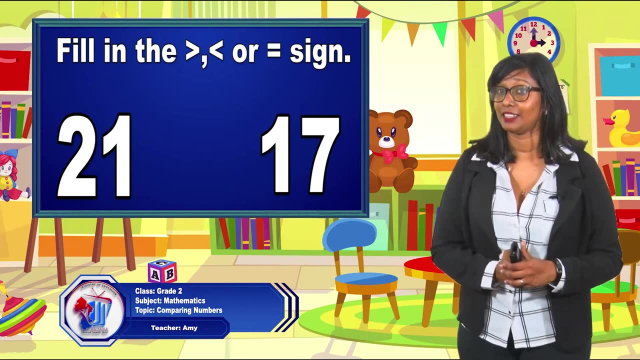 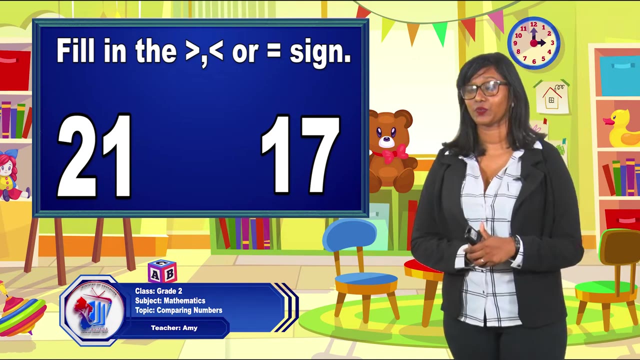 remember, the mouth of the alligator will be open to the bigger number and we use the equal sign when we're talking about the same number. so the first one: 21, 17, 21 and 17. which sign must we use? i'm giving you one minute to work that one and then we're going to discuss. 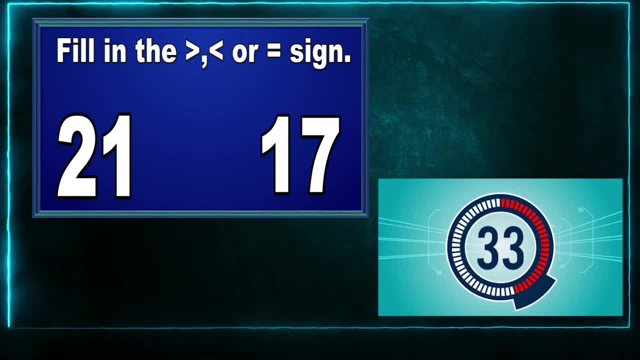 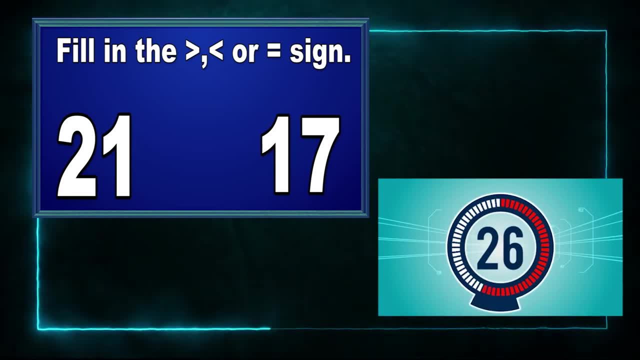 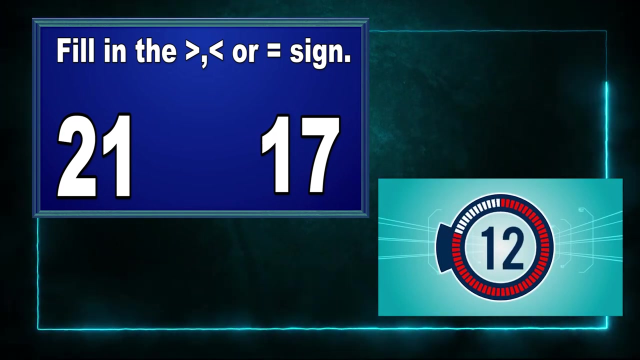 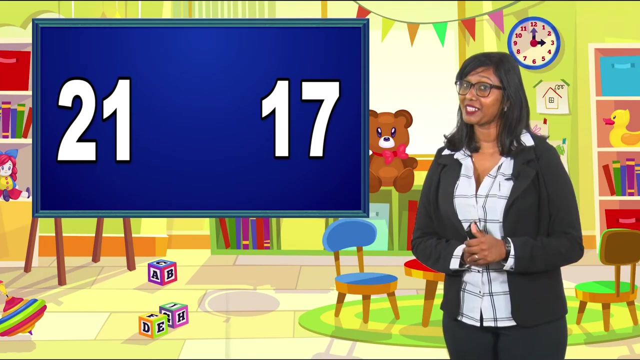 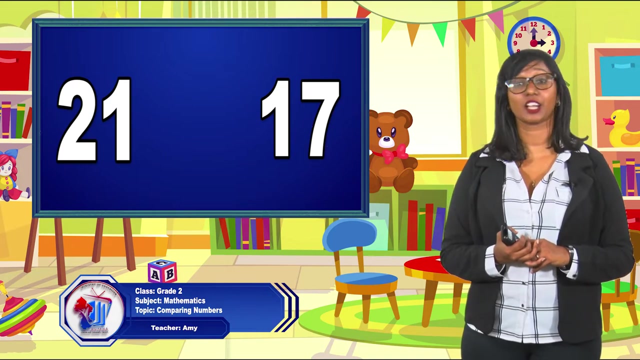 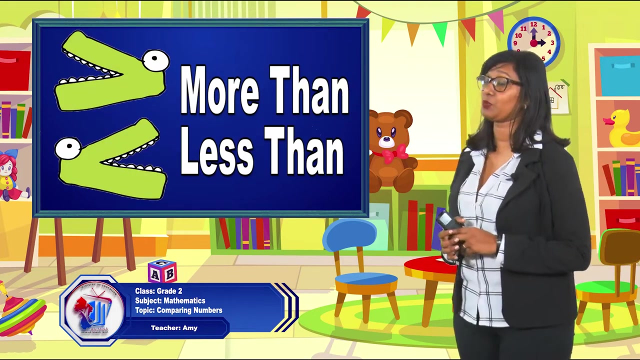 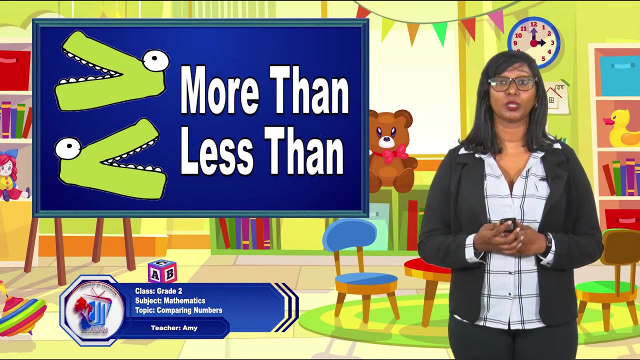 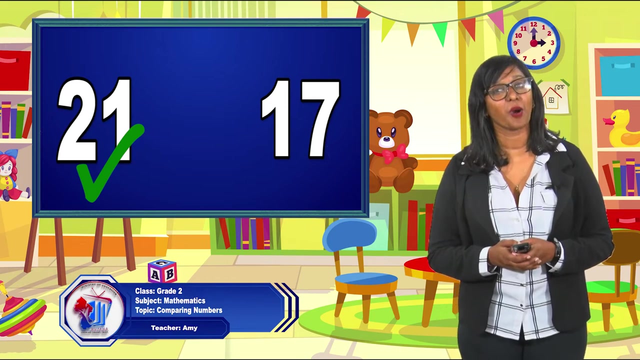 so okay, time's up. let's see 21 and 17. those two numbers are not the same, so therefore we cannot use our equal sign. so we have to choose between the more than sign and the less than sign. so the alligator's mouth will be open to the bigger number, and the bigger number here is 21. very good, 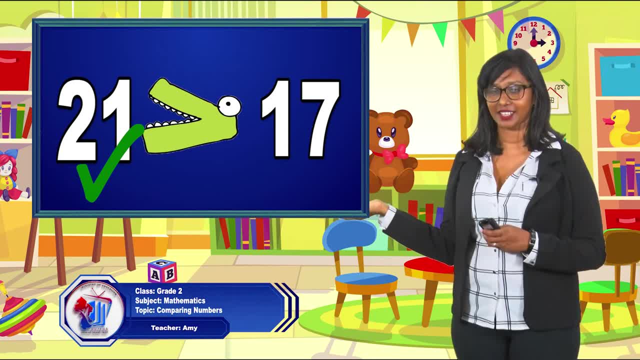 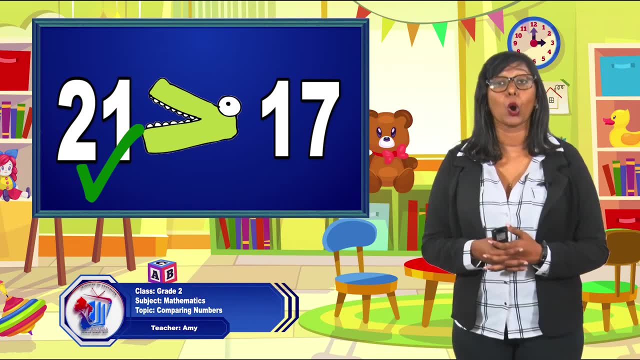 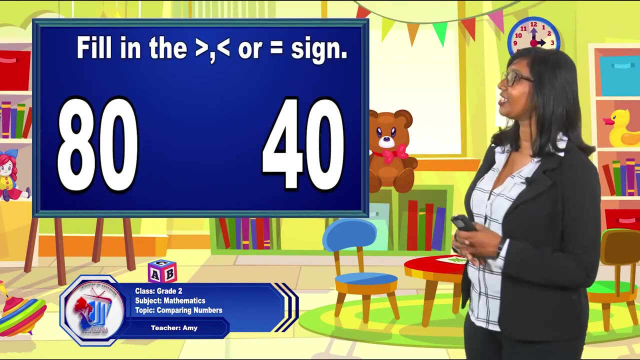 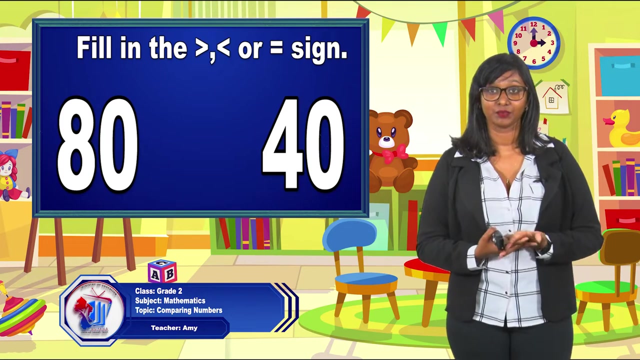 so therefore, we are going to use the more than sign, so we can say: 21 is bigger, greater or more than 17.. good job everyone. now let us move on to number two. number two says 80 and 40.. 80 and 40. so if we're to compare these two numbers, which sign? 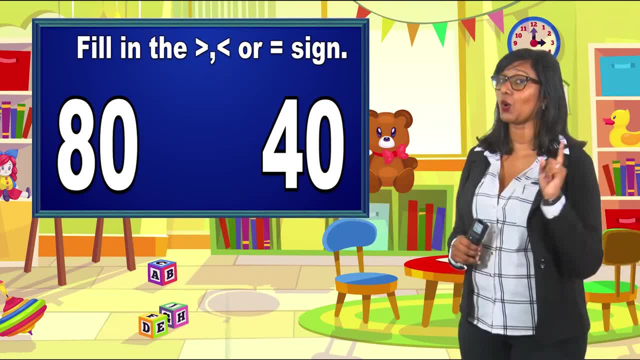 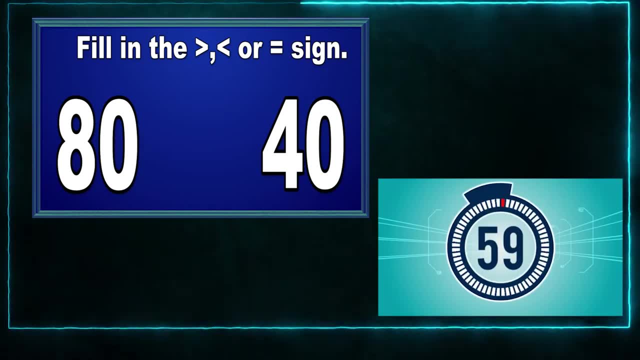 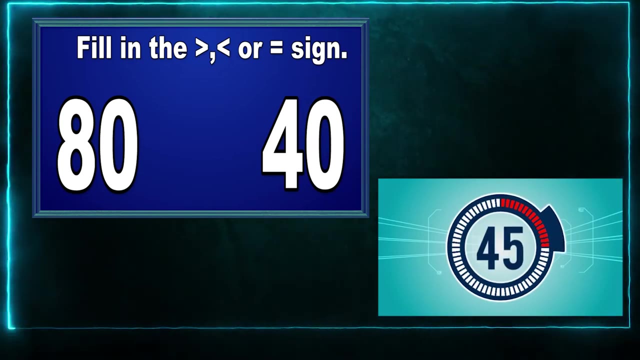 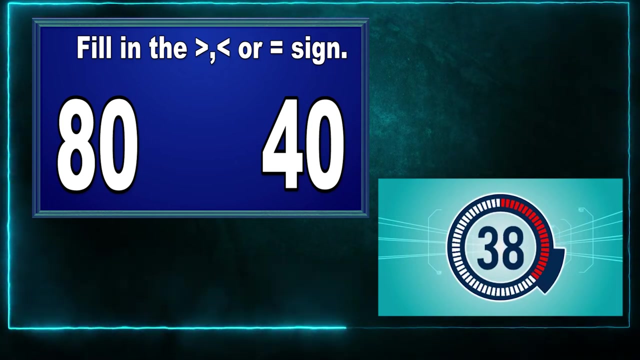 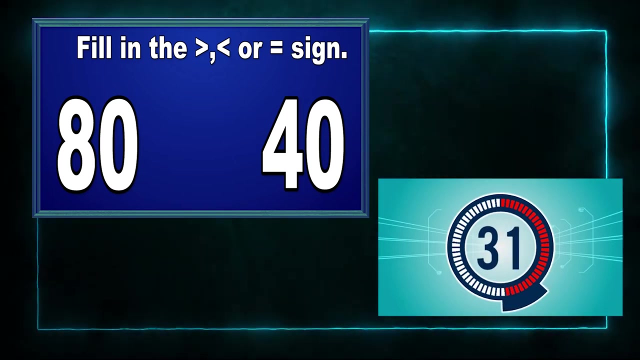 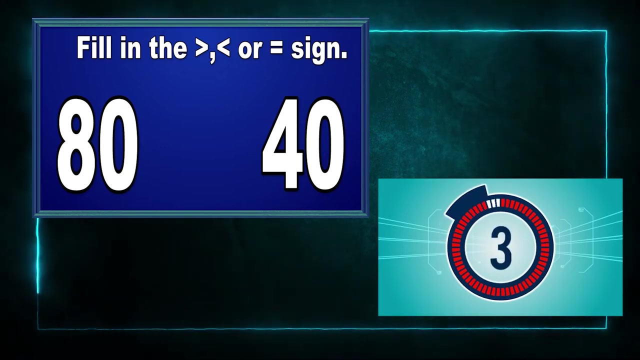 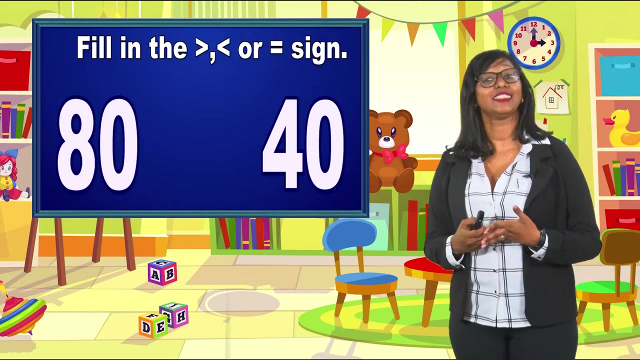 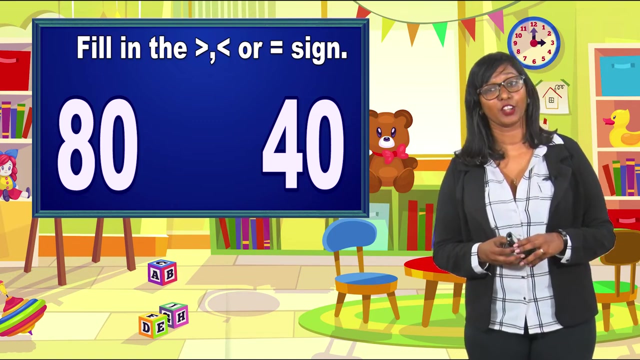 should we use. i'm giving you one minute to put in your sign and then we're going to discuss which sign you're going to trust the best for you, so you know whenever. okay, boys and girls, welcome back now. if we have 80 and 40, they are not the same. so if they are not the same, therefore, we 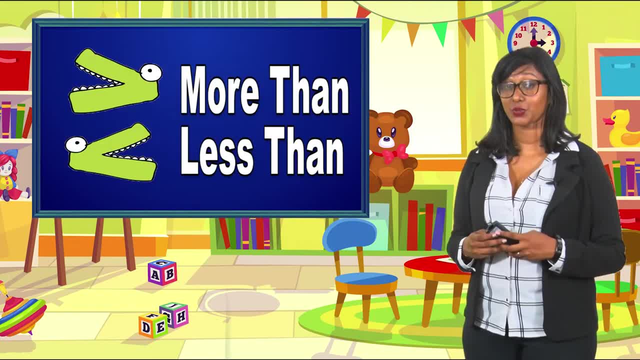 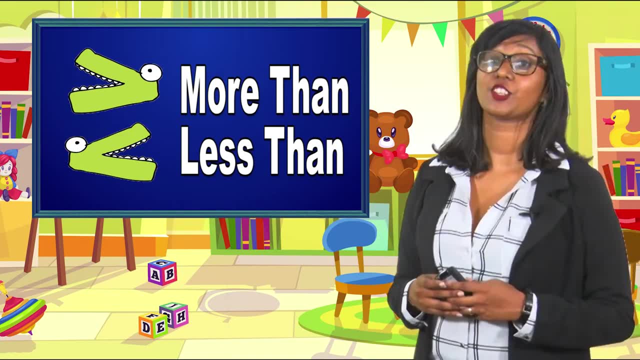 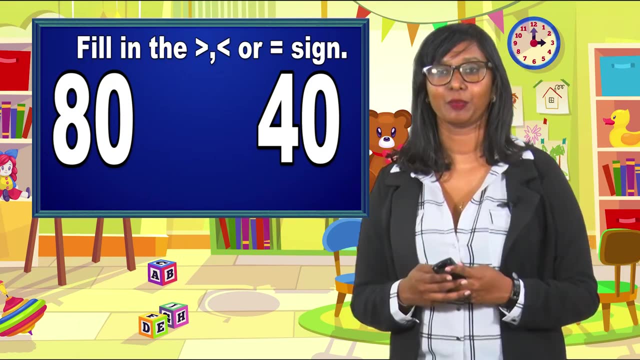 cannot use the equal sign, so we have to choose again from our more than sign and our less than sign. remember, the alligator is hungry and he wants to munch on the bigger number. so which one is the bigger number boys? I'm gonna ask the boys this question: which number is the bigger number boys? 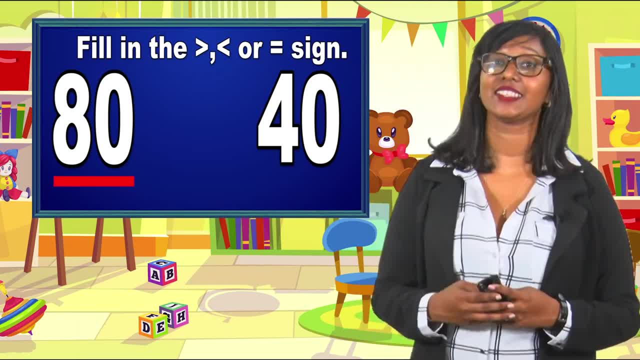 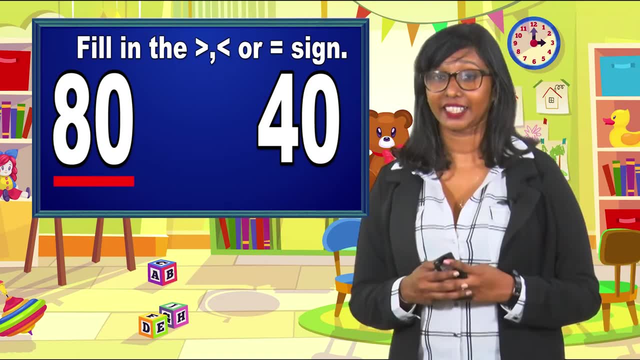 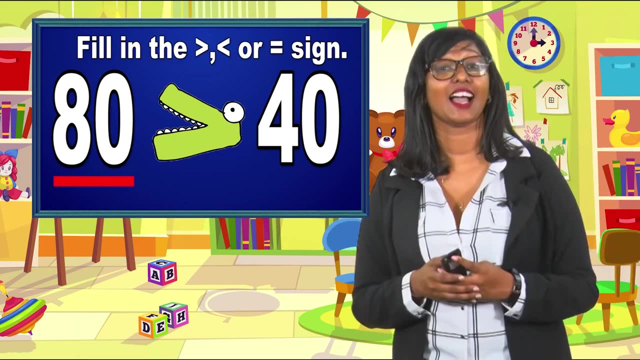 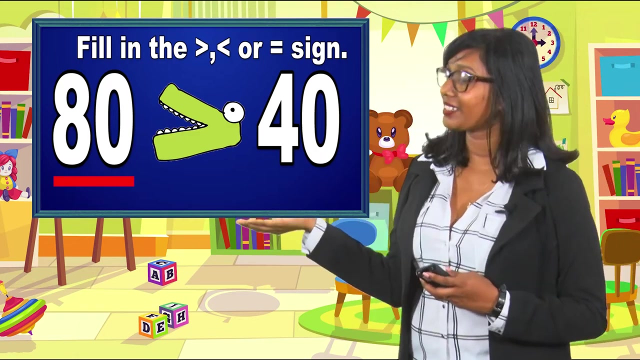 the bigger one, the bigger number is 80, very good. so girls tell me the mouth of the alligator will be open to 40 or 80, 80, very good. because the alligator likes the munch on big numbers, so we will use the more than sign and it reads: 80 is. 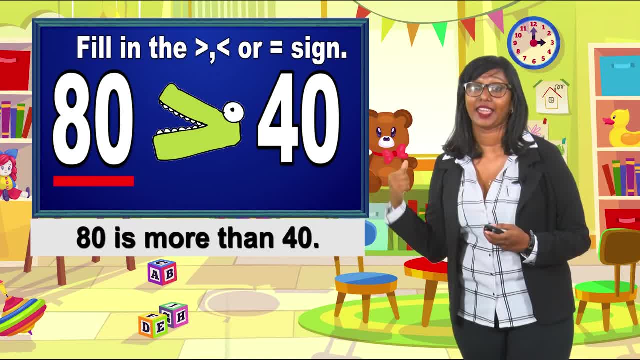 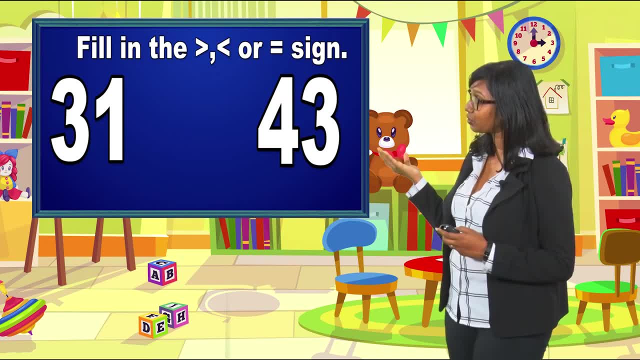 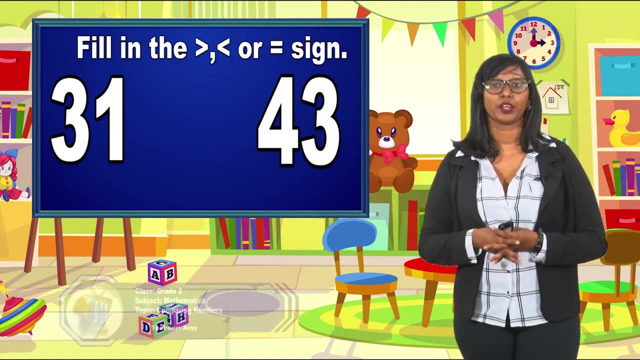 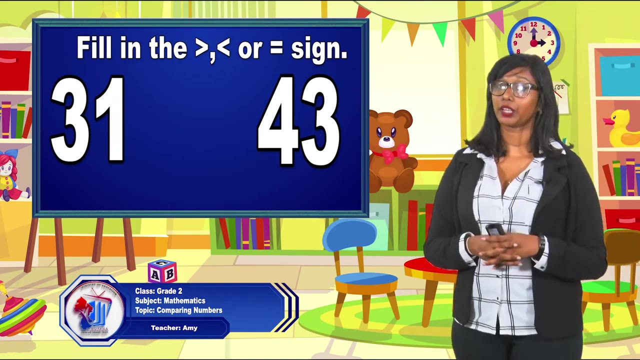 more than 40. 80 is more than 40. so I have another one here, number 3. number 3 says 31 and 43. so we are comparing the number 31 and 43. when we're comparing these two, remember the alligator wants to eat the bigger number. 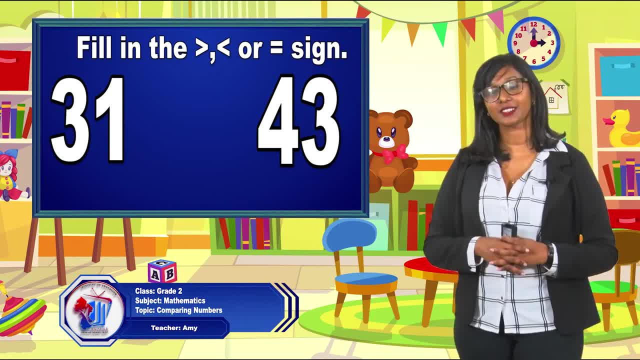 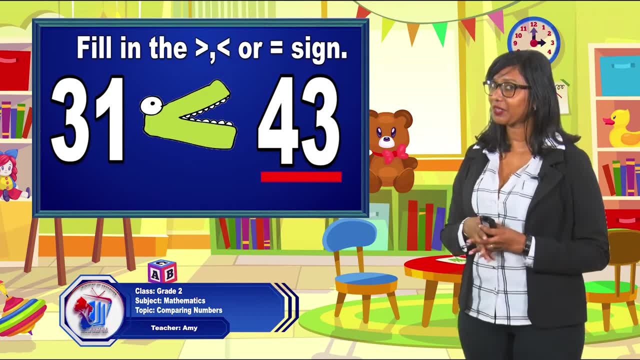 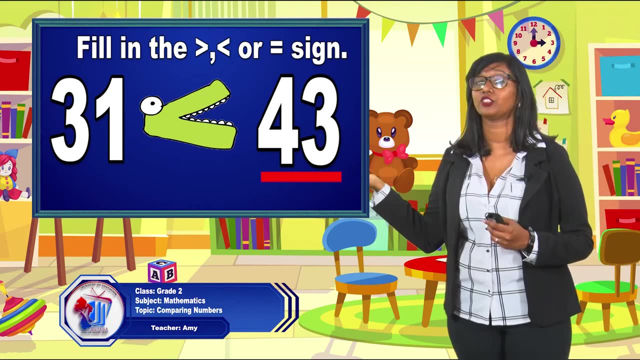 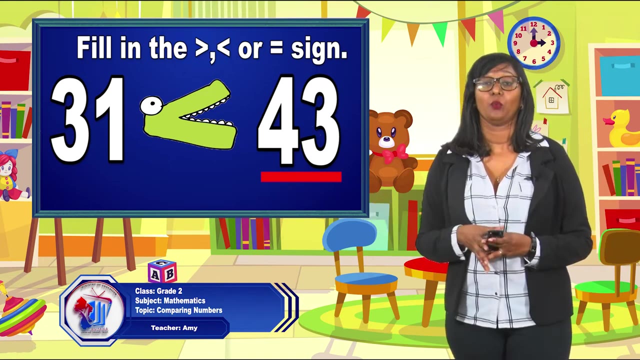 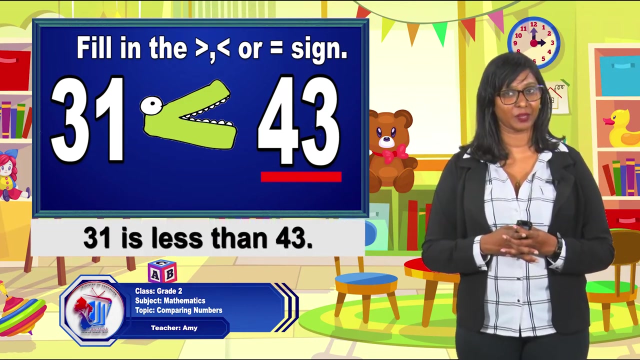 so which sign will we use? girls? we will use the less than sign. why do we use the less than sign? because the number 43 is bigger than 31, so the mouth of the alligator must be opened to 43. when we read this, it will read: 31 is less than 43. 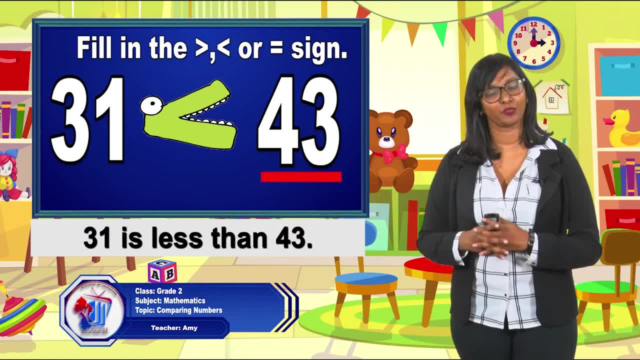 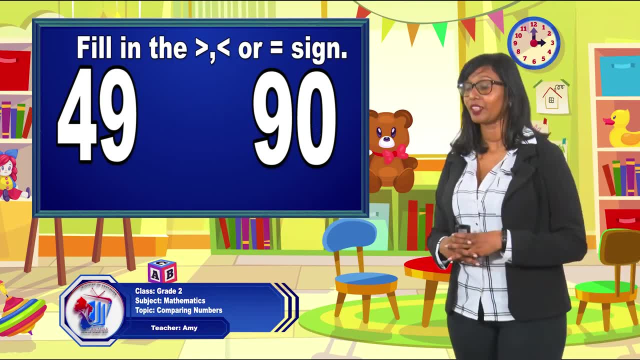 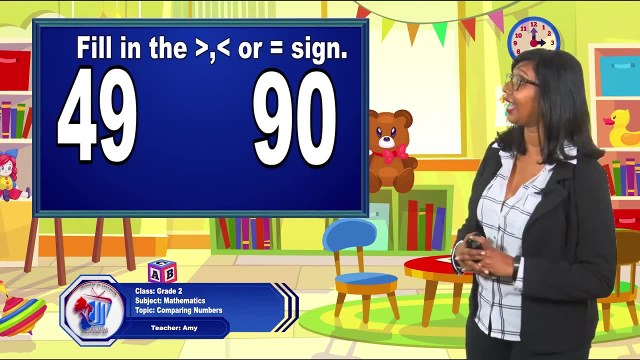 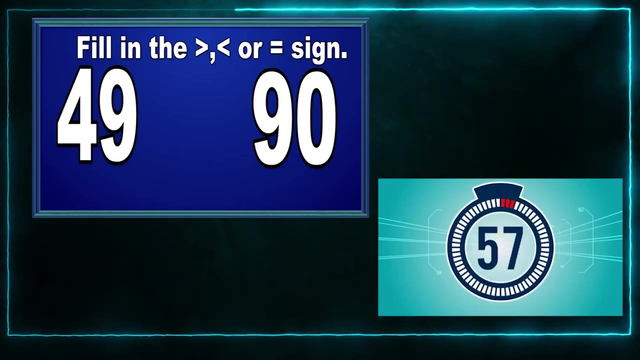 okay, you are doing a wonderful job thus far. so we have number four, our very last one, 49 when compared to 90. we are comparing 49 and 90. which sign must we use? okay, now the first letter to read 50 word. we will skip this. first, the biggest: 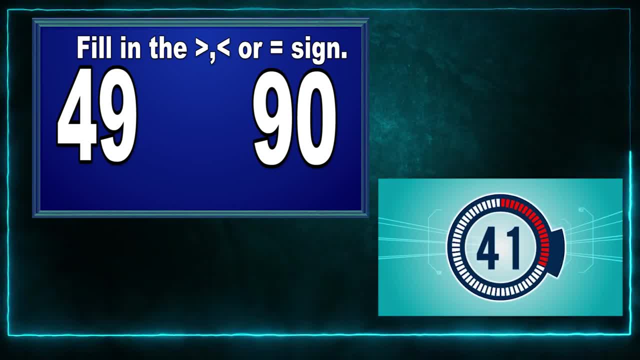 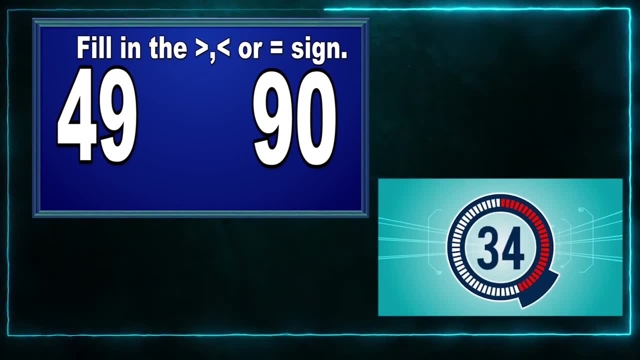 you will released all the other letters. Use the Q or R to see how you read the first few words. everything I sign is the enclosing. you can select other letters and it will be the independently of N, and N denotes your initial word. now the baby, and begin looking for a new word and then close the search items and open the. 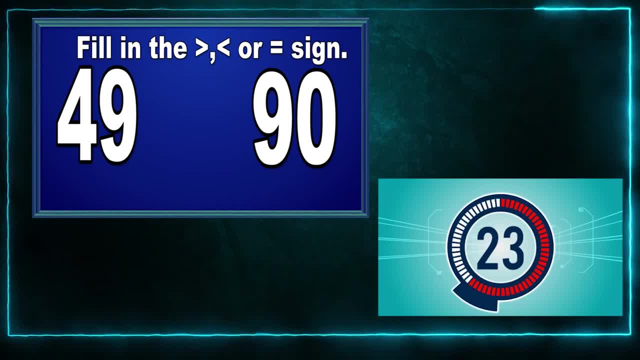 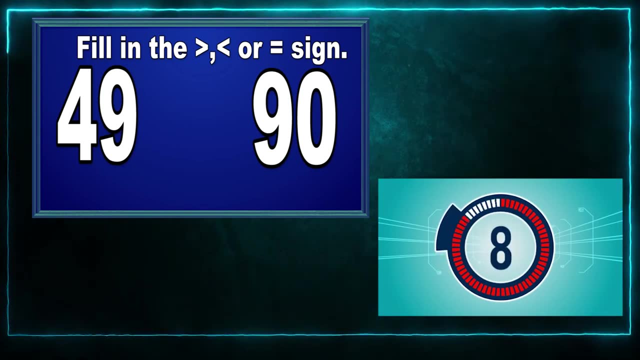 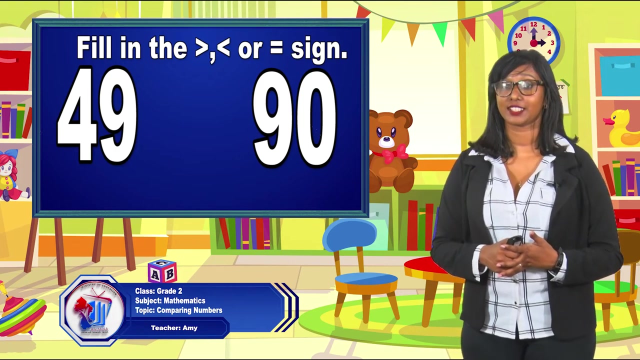 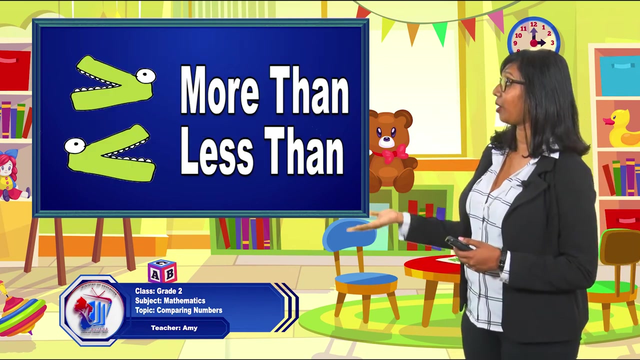 three, with all three letters, and then you will see that you get the first letter. These two numbers are not the same, So because they are not the same, we will not use the equal sign. So once again, we have to choose from the less than sign and the more than sign. 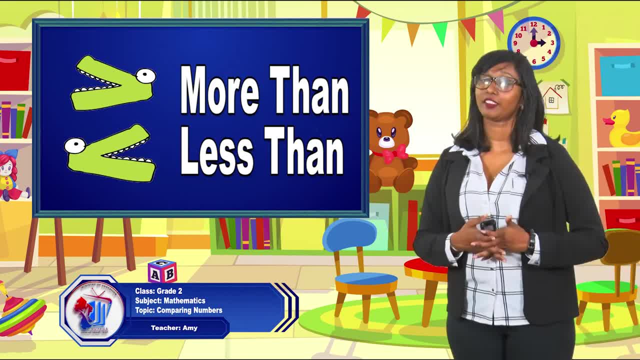 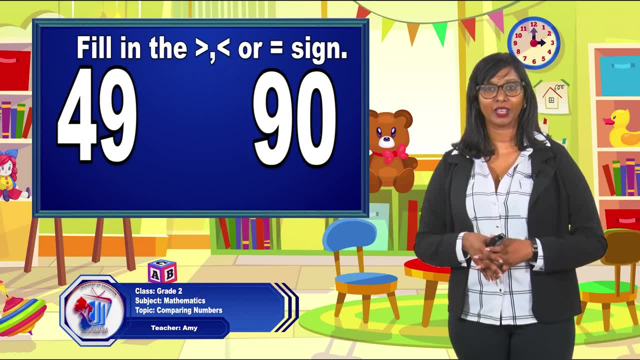 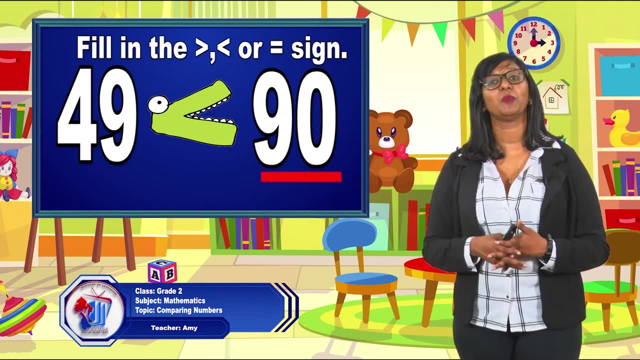 Remember, the alligator is very, very hungry and he will only eat the bigger number. So the mouth of the alligator will be open to 90.. Good job, The mouth of the alligator will be open. It will be open to 90..